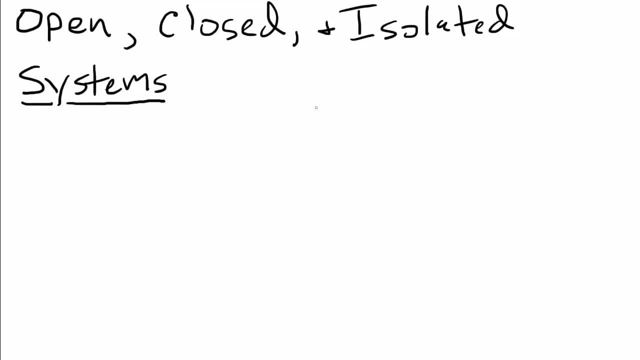 It's pretty simple, Basically, when we're thinking of thermochemistry or when we're thinking about energy, a lot of times it's very useful to think of there being two parts to the universe, And that is the thing that we're considering, which I'm going to represent. 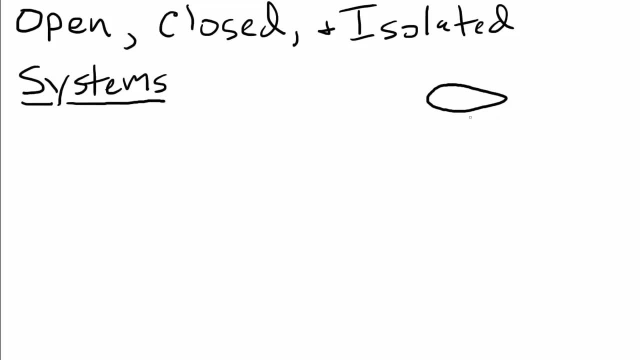 with this really deformed circle here that's called the system, And then everything else in the universe around it that we often will call the surroundings. So that's what a system is in terms of chemistry and thermochemistry and science, When we talk. 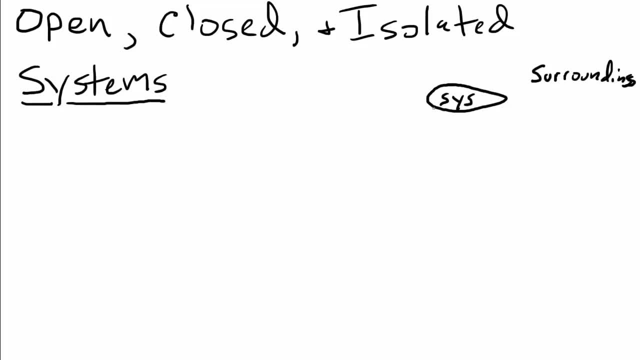 about a system. in science we're basically just talking about some part of the universe that's separate from everything else, And I know that seems really general and really kind of vague, but that's really basically all that it is. And so when we want to differentiate- 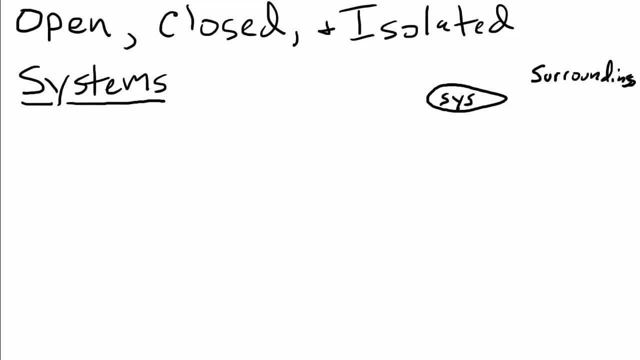 these three different things. we're going to start with the system And we're going to look at different types of systems: open, closed and isolated. It's really simple. This is going to be a pretty short lecture. Here's what it boils down to. We have to consider: 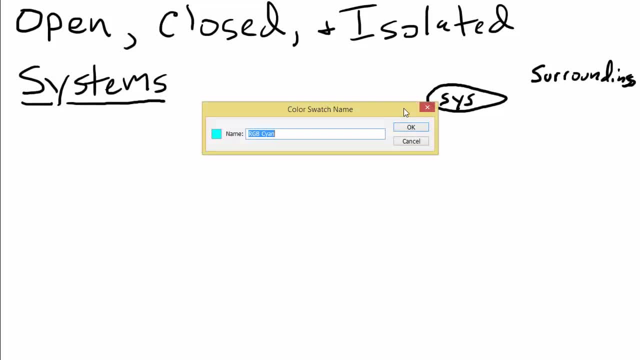 two things: matter and energy. So if matter is able to go into and out of a system and energy- let's see, I was going to use yellow, but I'm not sure that's going to show up very well- Purple color- And energy is also able to go into and out of the system, Then we call: 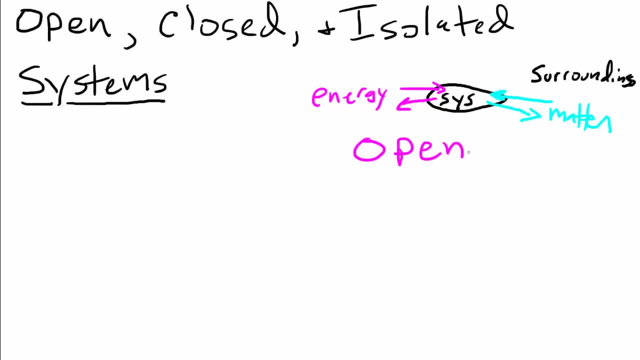 that an open system. So basically, there's nothing that's separating the system's matter and energy from that of the surroundings, and the system and the surroundings can exchange both of those things. That's called an open system. An example of an open system is if 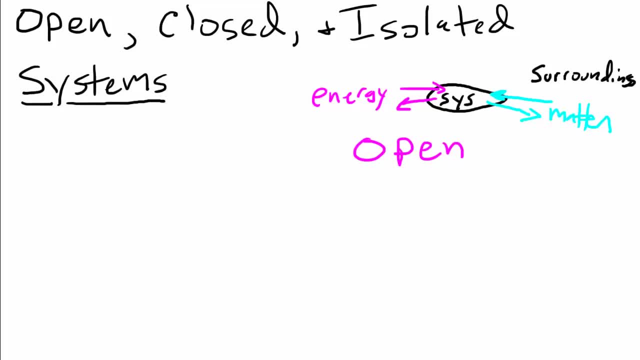 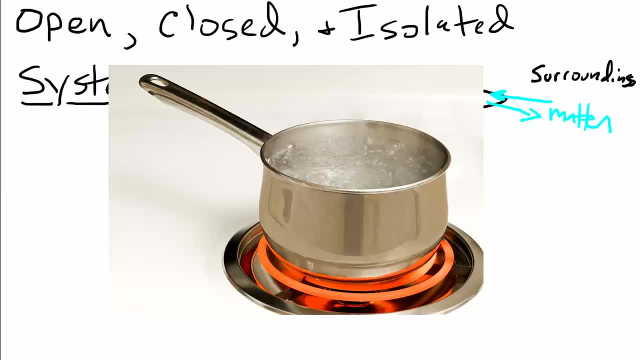 you have a pot of water on the stove Boiling, Maybe very similar to a pot like this. If you think about this, let's look at this picture and think about this a little bit. We're talking about energy and matter, right? So look at this red hot coil down here on the stovetop. That's adding energy. 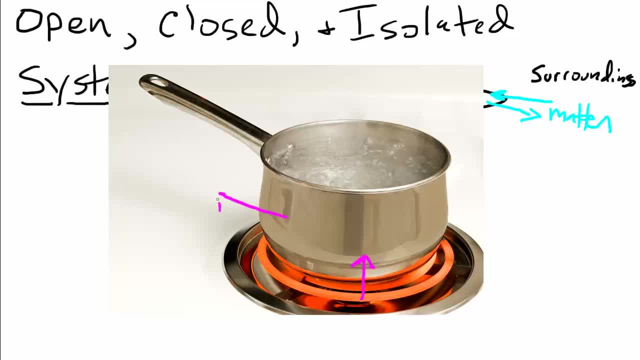 to the system. At the same time, this very hot pan is radiating heat energy out, and heat energy is rising out, convecting through the air as well. So not only is energy going into this system, it's also coming out of it. 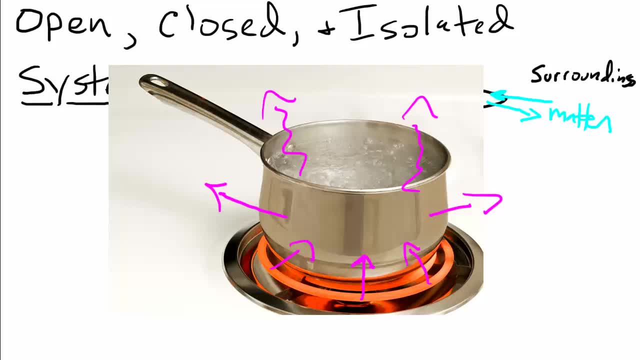 And at the same time there's no matter going into the system. But as the liquid water down here turns into gas, then we have matter leaving the system as well. So we have energy going into and coming out of the system and we have matter coming out of the system. This 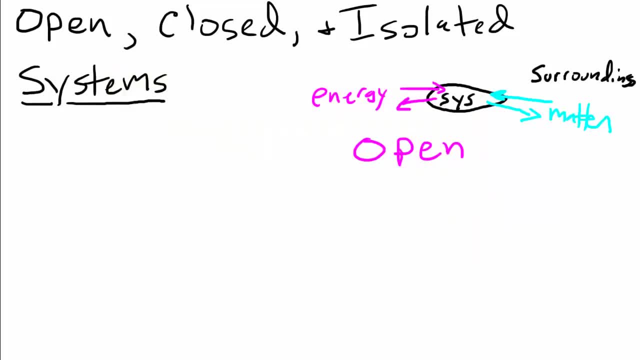 would be a great example of an open system. So the next type we're going to look at, then, is called closed, a closed system, And it's very similar to an open system. There's only one difference, So the energy can still go in and out. 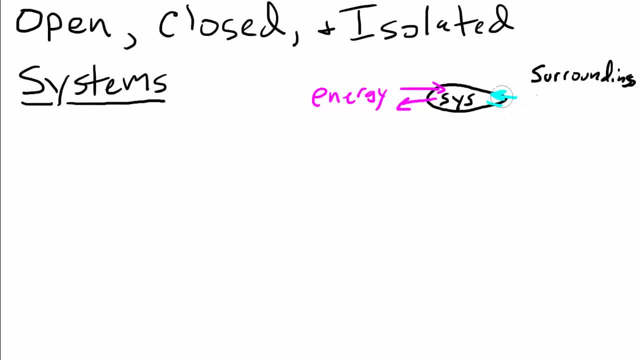 It's the matter that cannot go in and out. So if matter can't enter or leave a system, then it's called a closed system. So an open system, both matter and energy can go in and out, And in a closed system only energy can go in and out. 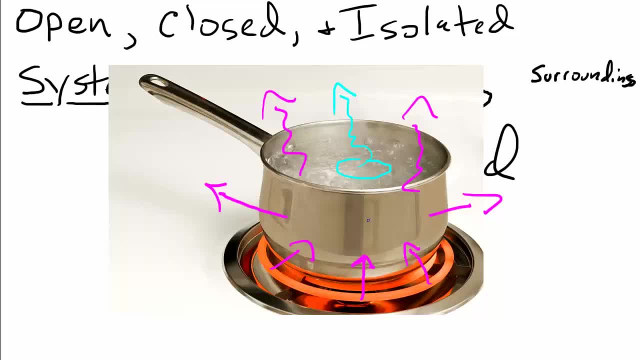 So an easy way to turn our pot here into a closed system is that if we had put a lid on it, Oops, what's going on here? Oops, so let's put a lid on this. I'm just going to draw a lid on here. 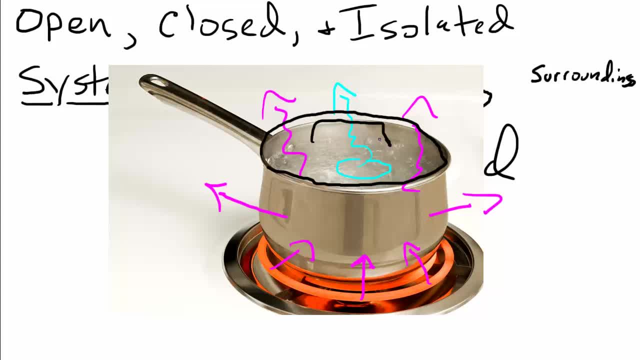 By drawing a lid on here. maybe it's got a handle. By drawing a lid on this, what we're basically doing is we're preventing the water from leaving now. So we've got energy entering and leaving the system, but this water back here can't. 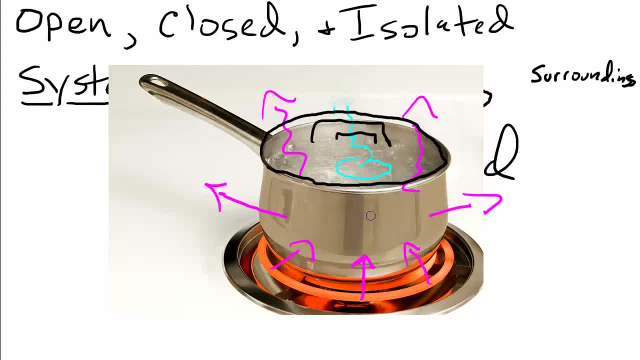 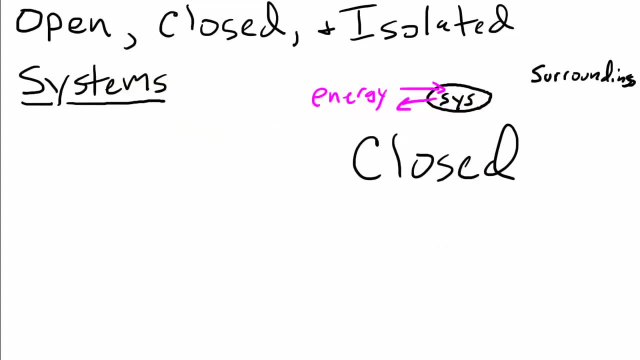 It's trapped inside, So the energy can still come in and out, but the water cannot, And so now we've turned our pot, which used to be an open system, into a closed system by sealing it off, And so then you can probably guess what the last one is the isolated system. 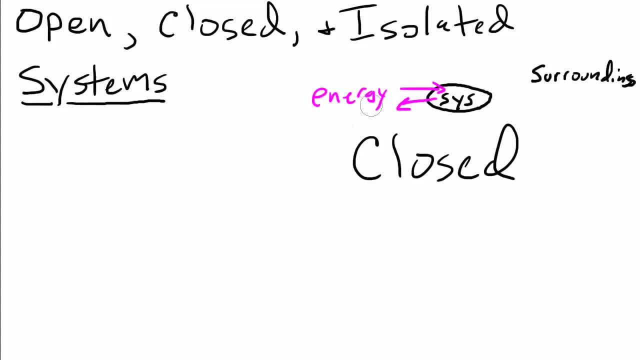 That's the most restrictive of the three and we're going to remove the energy now. So this is a system that's completely separated from the rest of its surroundings. Neither matter nor energy can go into or come out of it. It's completely closed.